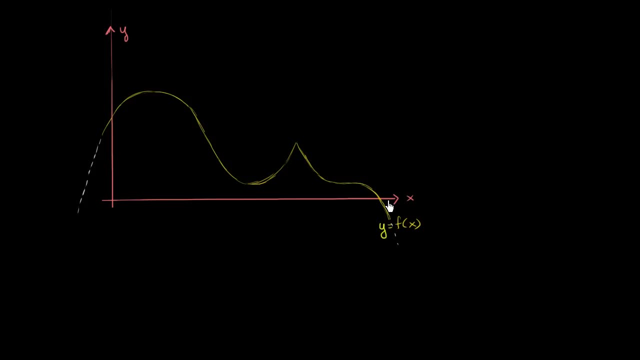 as x becomes more and more negative and lower and lower and lower as x goes beyond the interval that I've depicted right over here. So what is the maximum value that this function takes on? Well, we can eyeball that It looks like it's at this point. 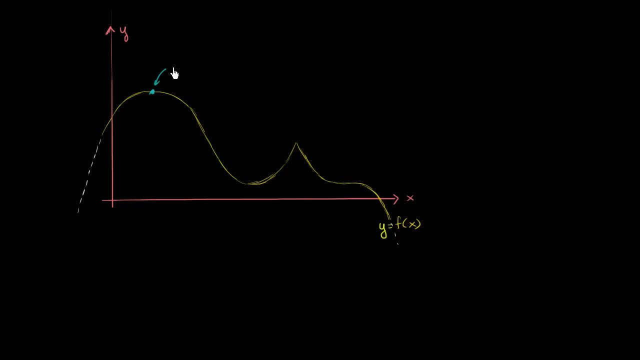 It looks like it's at that point right over there, So we would call this a global maximum. The function never takes on a value larger than this, So we could say that we have a global maximum at the point x0, because f of x0 is greater than or equal to f of x. 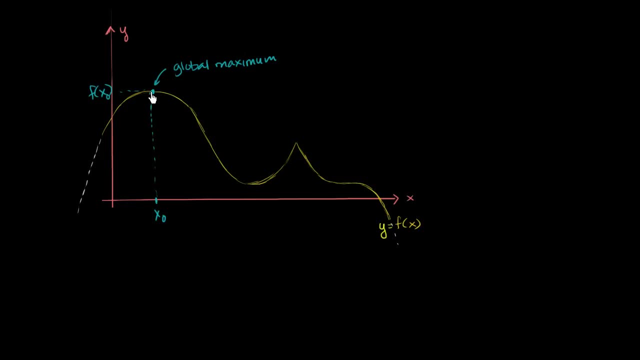 for any other x in the domain, And that's pretty obvious when you look at it like this. Now, do we have a global maximum? Do we have a global minimum? point, the way that I've drawn it. Well, no, This function can take on arbitrarily negative values. 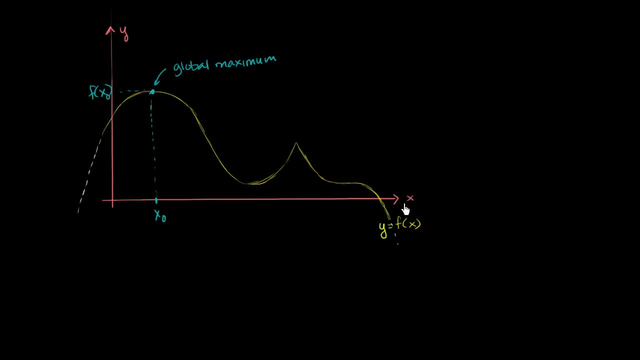 It approaches negative infinity as x approaches negative infinity. It approaches negative infinity as x approaches positive infinity. So we have- let me write this down, we have no global minimum. Now let me ask you a question: Do we have local minima or local maximum? 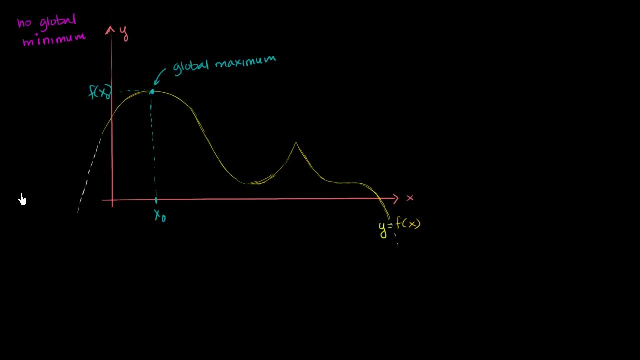 What? When you say minima, it's just the plural of minimum And maxima is just the plural of maximum. So do we have a local minima here or local minimum here? Well, a local minimum, you could imagine. 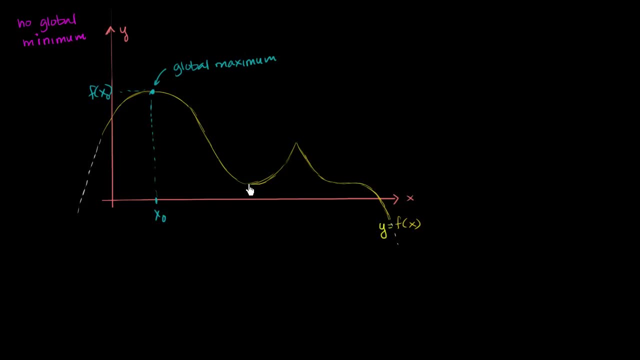 means that that value of the function at that point is lower than the points around it. So right over here it looks like we have a local minimum And I'm not giving you a very rigorous definition here. But one way to think about it is we 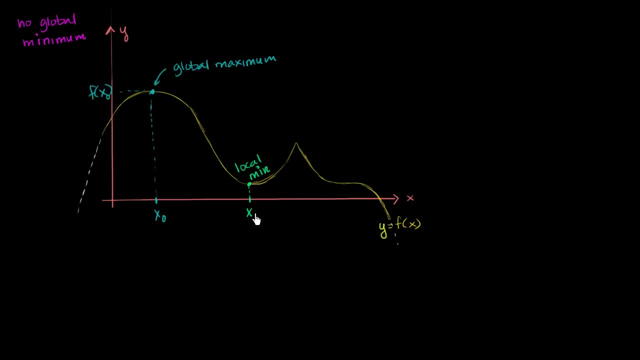 can say that we have a local minimum, And the local minimum point at x1 is if we have a region around x1 where f of x1 is less than an f of x for any x in this region right over here And it's pretty easy to eyeball too. 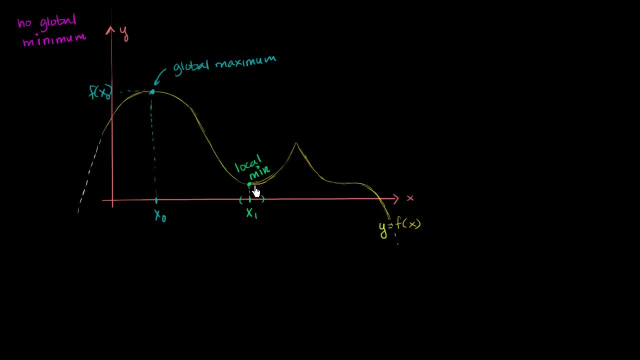 This is a low point for any of the values of f around it right over there. Now, do we have any other local minima? Well, it doesn't look like we do. Now, what about local maxima? Well, this one right over here. let me do it in. 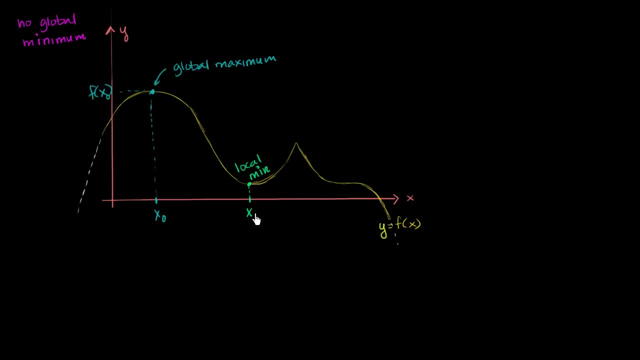 can say that we have a local minimum, And the local minimum point at x1 is if we have a region around x1 where f of x1 is less than an f of x for any x in this region right over here And it's pretty easy to eyeball too. 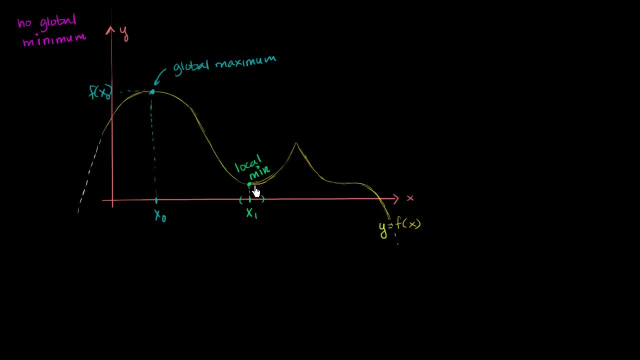 This is a low point for any of the values of f around it right over there. Now, do we have any other local minima? Well, it doesn't look like we do. Now, what about local maxima? Well, this one right over here. let me do it in. 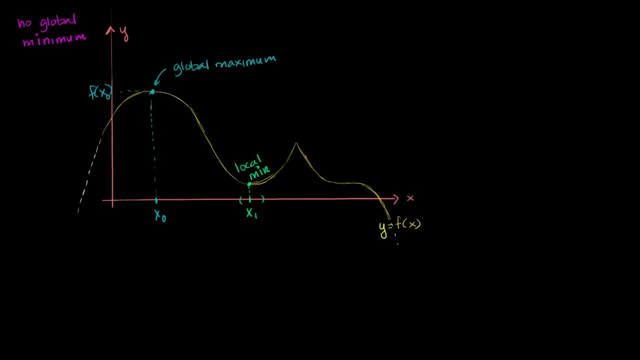 Let me do it. Let me do it in purple. I don't want to get people confused. actually, Let me do it in this color. This point right over here looks like a local maximum. Local, not lox. That would have to deal with salmon. 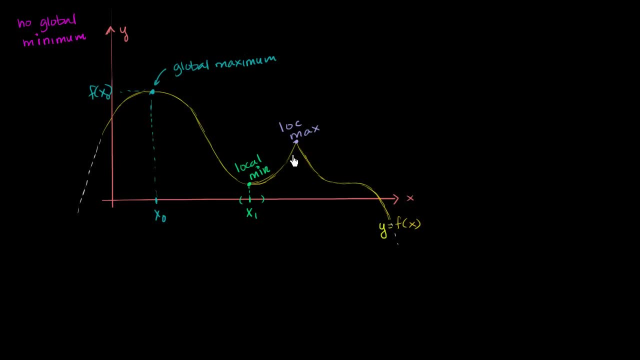 Local maximum right over there. Local maximum. So we could say at the point x1,, at the point x2, or we have a local maximum point at x2, because f of x2 is larger. It's larger than f of x for any x around a neighborhood. 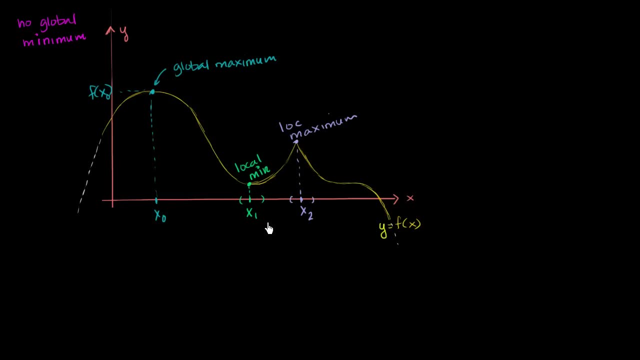 around x2.. I'm not being very rigorous, but you can see it just by looking at it. So that's fair enough. We've identified all of the maxima and minima, often called the extrema, for this function. Now how can we identify those if we? 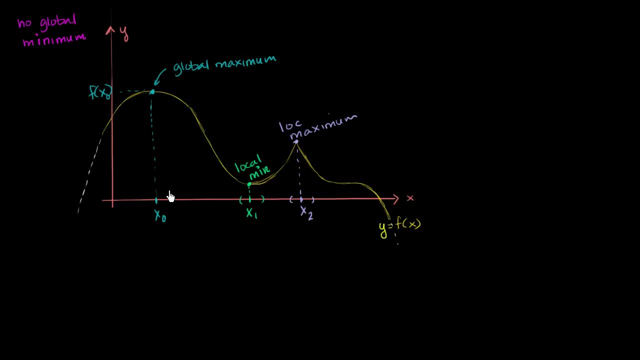 knew something about the derivative of the function. Well, let's look at the derivative at each of these points. So at this first point, right over here, if I were to try to visualize the tangent, let me do that in a better color than brown. 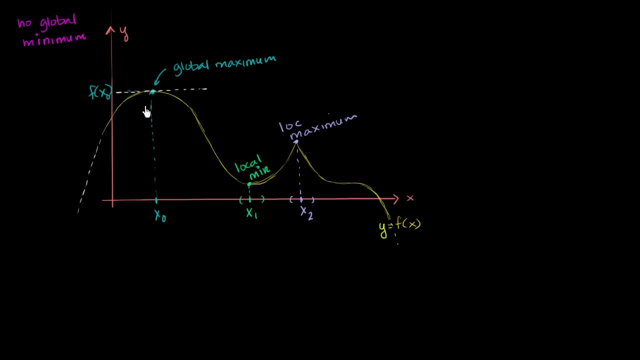 If I were to try to visualize the tangent line, it would look something like that: So the slope here is 0.. So we would say that f prime of x0 is equal to 0.. The slope of the tangent line at this point is 0. 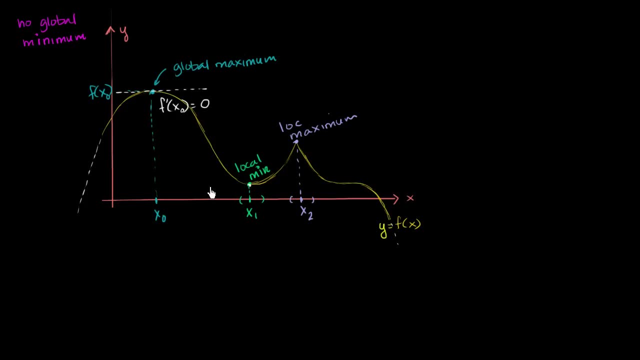 What about over here? Well, once again the tangent line would look something like that. So once again we would say: f prime at x1 is equal to 0.. What about over here? Well, here the tangent line is actually not well-defined. 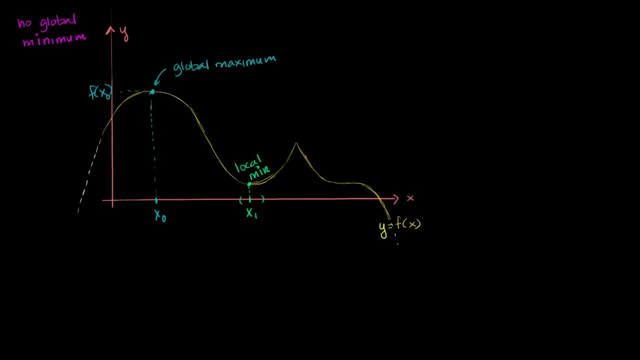 Let me do it. Let me do it in purple. I don't want to get people confused. actually, Let me do it in this color. This point right over here looks like a local maximum. Local, not lox. That would have to deal with salmon. 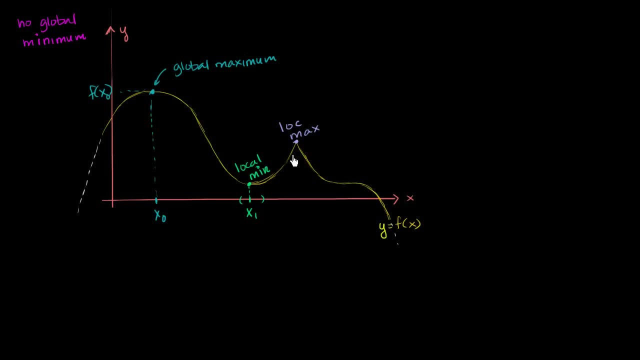 Local maximum right over there. Local maximum. So we could say at the point x1,, at the point x2, or we have a local maximum point at x2, because f of x2 is larger. It's larger than f of x for any x around a neighborhood. 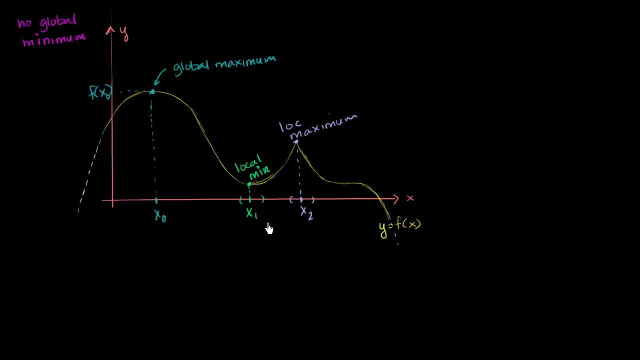 around x2.. I'm not being very rigorous, but you can see it just by looking at it. So that's fair enough. We've identified all of the maxima and minima, often called the extrema, for this function. Now how can we identify those if we? 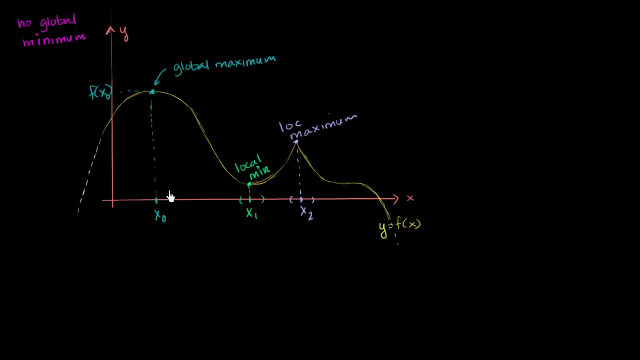 knew something about the derivative of the function. Well, let's look at the derivative at each of these points. So at this first point, right over here, if I were to try to visualize the tangent, let me do that in a better color than brown. 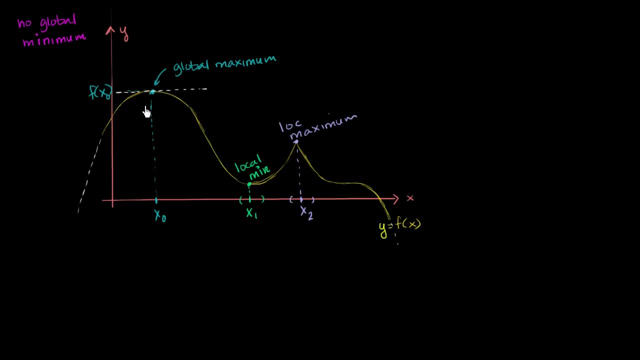 If I were to try to visualize the tangent line, it would look something like that: So the slope here is 0.. So we would say that f prime of x0 is equal to 0.. The slope of the tangent line at this point is 0. 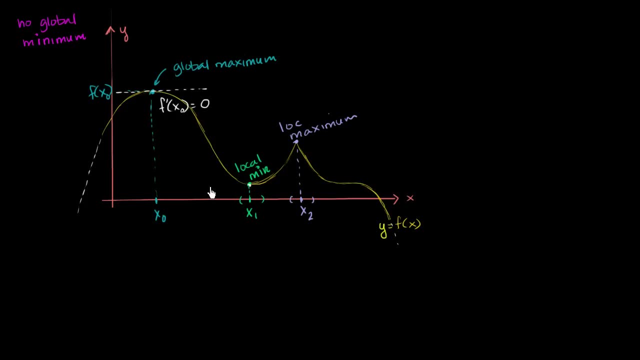 What about over here? Well, once again the tangent line would look something like that. So once again we would say: f prime at x1 is equal to 0.. What about over here? Well, here the tangent line is actually not well-defined. 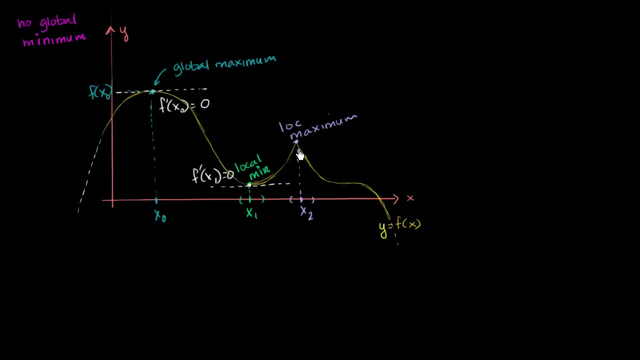 We have a positive slope going into it and then it immediately jumps to being a negative slope. So over here, f prime of x2 is not defined, Let me just write undefined. So we have an interesting- and once again I'm not rigorously- 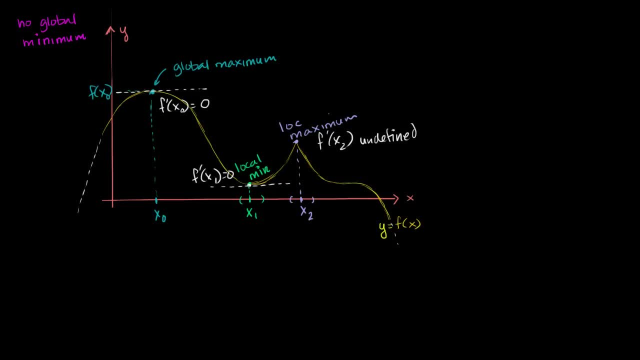 proving it to you, I just want you to get the intuition here- We see that if we have some type of extrema- and we're not talking about when we're at 0. We're talking about when x is at an endpoint of an interval- 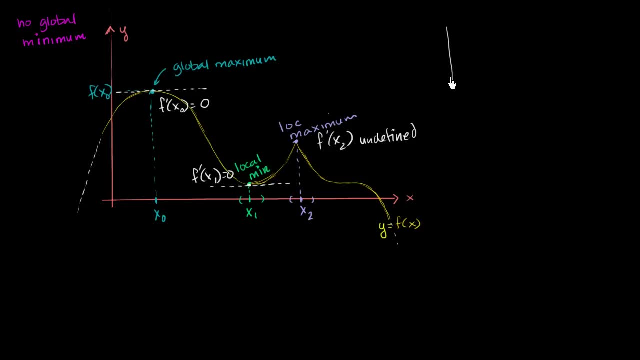 Just to be clear what I'm talking about. when I'm talking about x as an endpoint of an interval, we're saying: let's say that the function is, let's say we have an interval from there, So let's say a function starts right over there. 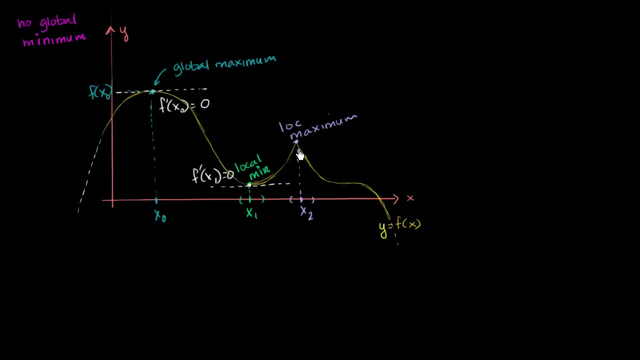 We have a positive slope going into it and then it immediately jumps to being a negative slope. So over here, f prime of x2 is not defined, Let me just write undefined. So we have an interesting- and once again I'm not rigorously- 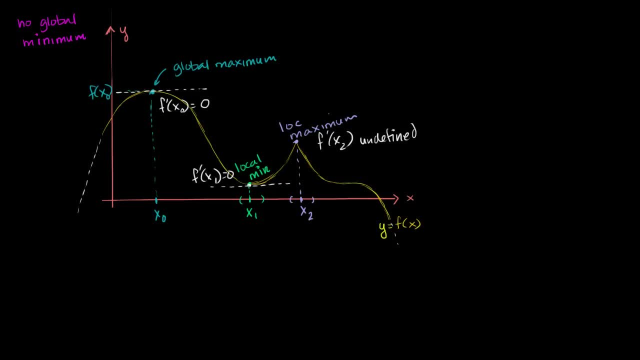 proving it to you, I just want you to get the intuition here- We see that if we have some type of an extrema- and we're not talking about when we're at 0. We're talking about when x is at an endpoint of an interval- 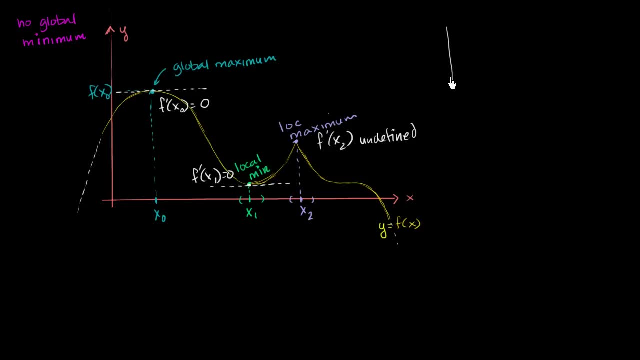 Just to be clear what I'm talking about. when I'm talking about x as an endpoint of an interval, we're saying: let's say that the function is, let's say we have an interval from there, So let's say a function starts right over there. 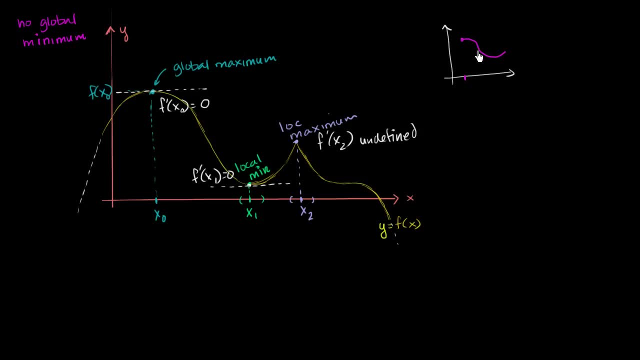 and then keeps going. This would be a maximum point, but it would be an endpoint. We're not talking about endpoints right now. We're talking about when we have points in between or when our interval is infinite. So we're not talking about points like that. 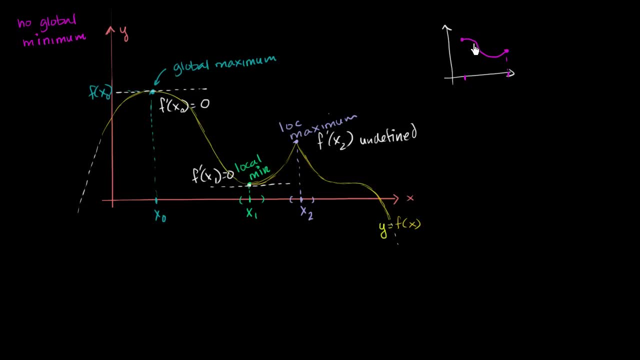 Or points like this. We're talking about the points in between. So if you have a point inside of an interval, it's going to be a minimum or maximum, And we see the intuition here. If you have nonendpoint, nonendpoint, nonendpoint, min. 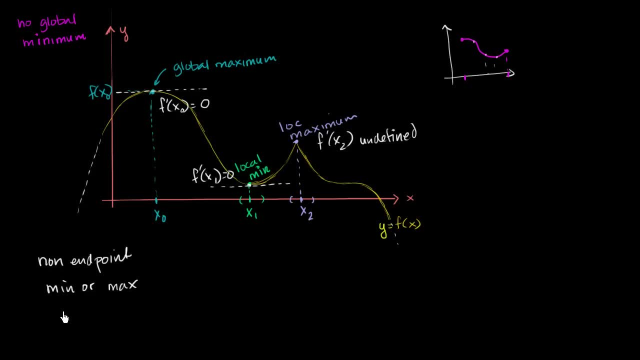 or max, min or max at, let's say, x is equal to a. So if you know that you have a min, minimum or maximum point at some point, x is equal to a and x isn't the endpoint of some interval. 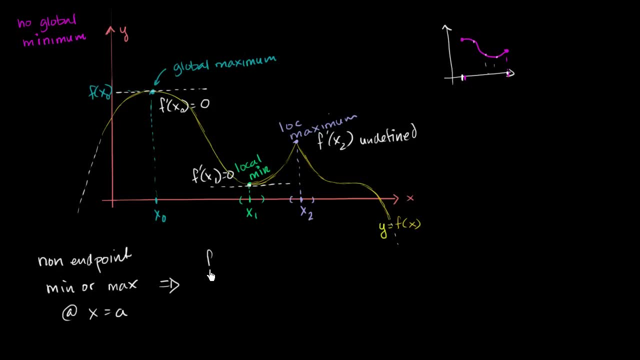 This tells you something interesting, or at least we have the intuition. We see that the derivative at x is equal to a is going to be equal to 0, or the derivative at x is equal to a is going to be undefined. And we see that in each of these cases. 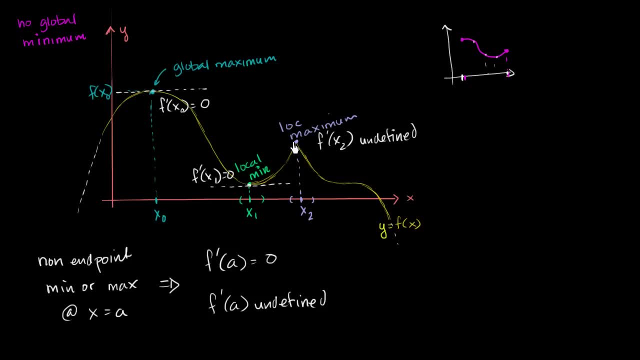 Derivative is 0, derivative is 0.. Derivative is undefined. And we have a word for these points where the derivative is either 0 or the derivative is undefined. We call them critical points. So, for the sake of this function, the critical points. 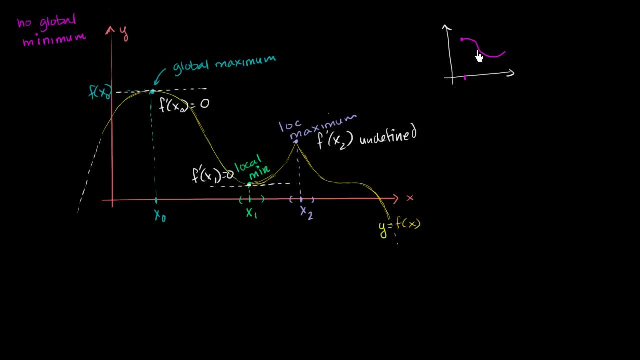 and then keeps going. This would be a maximum point, but it would be an endpoint. We're not talking about endpoints right now. We're talking about when we have points in between or when our interval is infinite. So we're not talking about points. 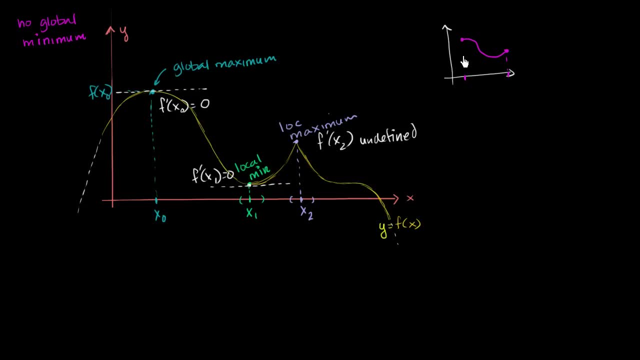 like that or points like this. We're talking about the points in between. So if you have a point inside of an interval, it's going to be a minimum or maximum, And we see the intuition here. If you have so non-endpoint. 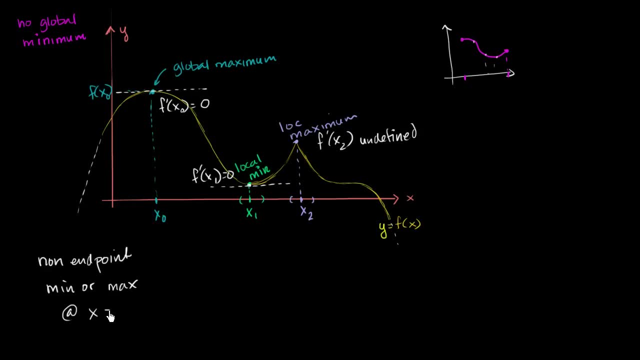 Min or max at, let's say, x is equal to a Right. So if you know that you have a minimum or maximum point at some point, x is equal to a and x isn't the end point. x isn't the end point of some interval. 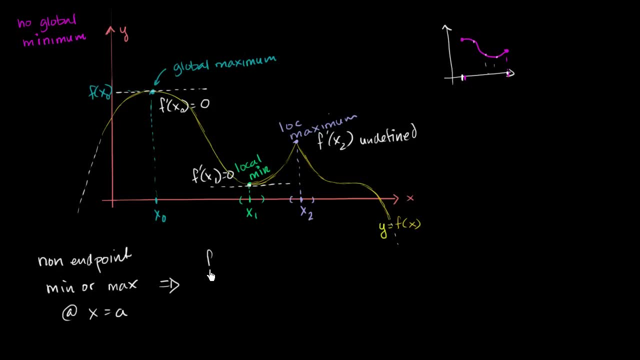 this tells you something interesting, or at least we have the intuition. We see that the derivative at x is equal to a is going to be equal to 0, or the derivative at x is equal to a is going to be undefined. And we see that in each of these cases. 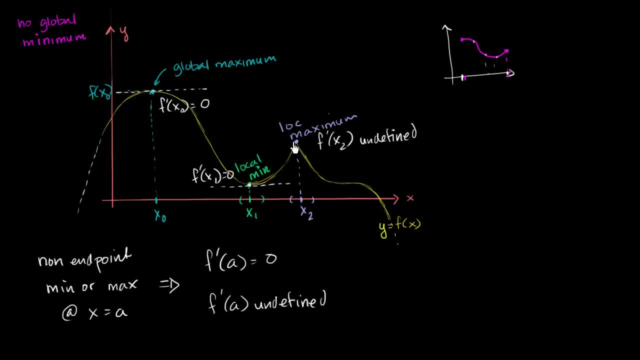 Derivative is 0, derivative is 0.. Derivative is undefined. And we have a word for these points where the derivative is either 0 or the derivative is undefined: We call them critical points. So, for the sake of this function, 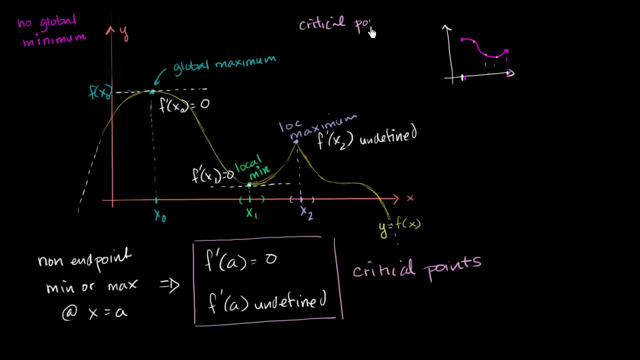 the critical points are: if we could include x sub 0,, we could include x sub 2.. We could include x sub 1.. At x sub 0 and x sub 1,, the derivative is 0. And x sub 2, where the function is undefined. 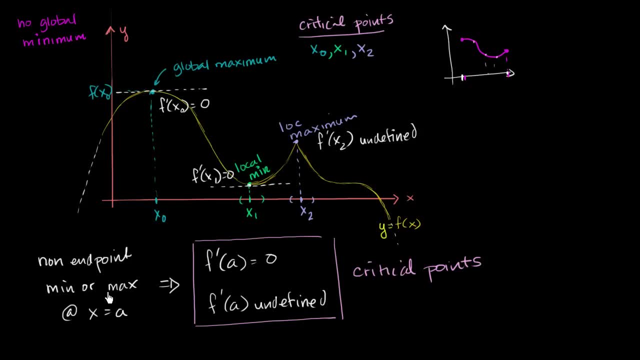 Now. so if we have a non-end point, minimum or maximum point, then it's going to be a critical point. But can we say it the other way around? If we find a critical point where the derivative is 0, or the derivative is undefined, is that? 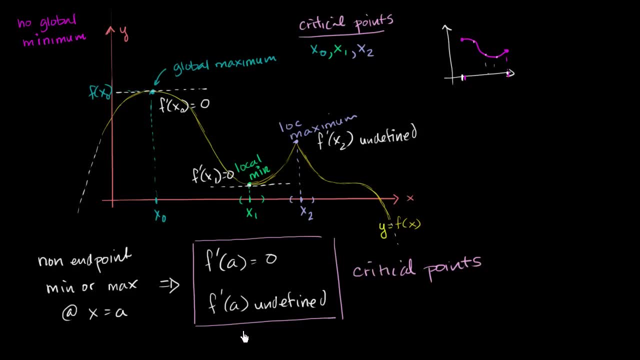 going to be a maximum or minimum point, And to think about that, let's imagine, let's imagine this point right over here. So let's call this x, sub 3.. If we look at the tangent line right over here, if we look at the slope right over here,